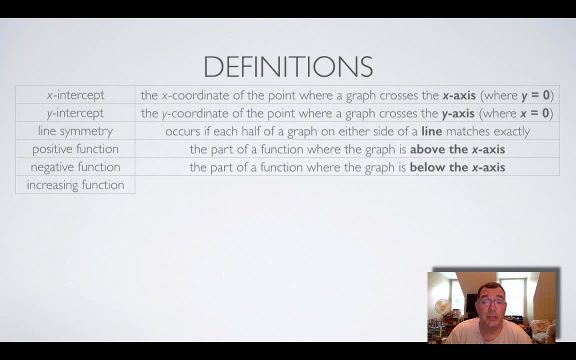 We talk about increasing functions and decreasing functions, and when we do that, we are reading the graph from left to right. We never read it from right to left. So when I talk about increasing and decreasing, I talk about what's happening as the graph goes to the right. So if the graph goes up and to the 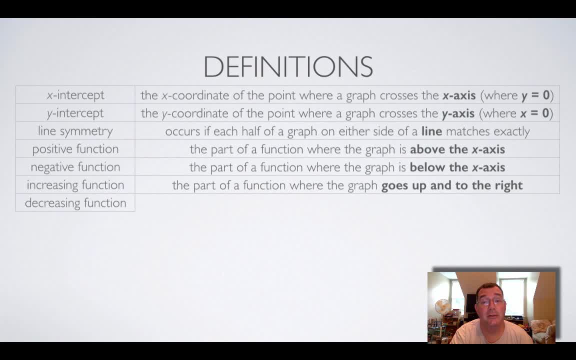 right, that is an increasing function, and if the graph goes down and to the right, that is a decreasing function. So there's the difference between those two. A relative maximum is any part of the graph where it reaches like a high value, like a hill, and then decreases after it. 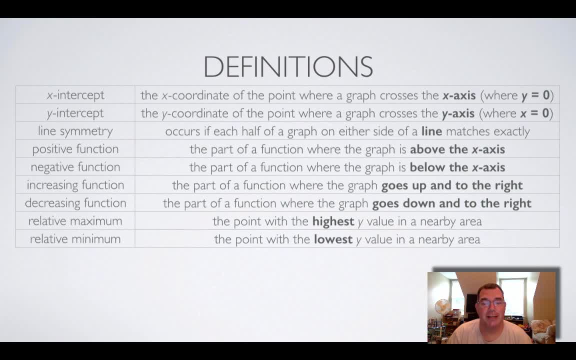 And a relative minimum is where there's like a valley. it reaches a low point and then comes back up. We're going to see visual examples of all of these. End behavior is what's happening as the graph goes very, very left off of the actual graph that you can see and very 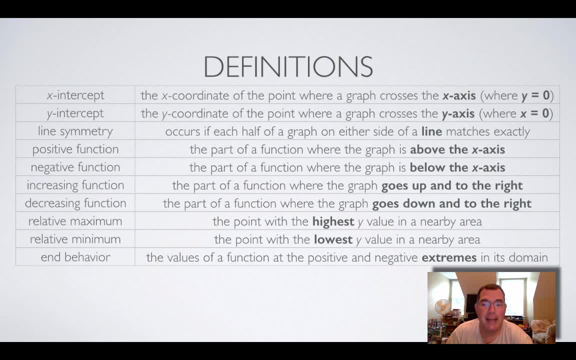 very right off of the graph. So it's just looking at what's happening as you go very, very far into. x equals negative infinity and x equals positive infinity is what they like to call it. So let's look at specifically the first few of those intercepts, positives and negatives. So 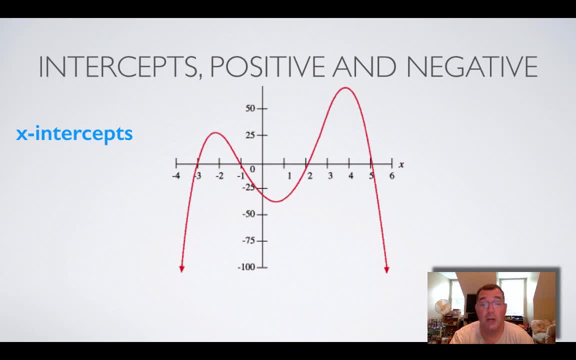 the x-intercepts on this graph are where the red curve crosses the x-axis, that horizontal axis, and there's four of those labeled with blue points. The y-intercept is going to be where it crosses the y-axis, which is that one pink point right there. The graph is positive anywhere that it goes above. 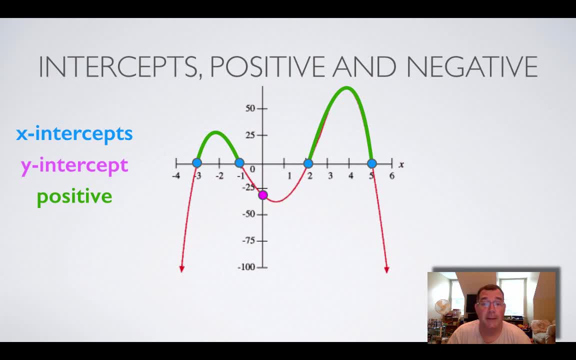 the x-axis, so I've labeled those with green parts of the curve. Those are the spots on the graph that are above the x-axis, and then the negative spots are obviously everywhere else where it's below the x-axis, And so what you should notice is that the green and the purple are always separated by a blue. 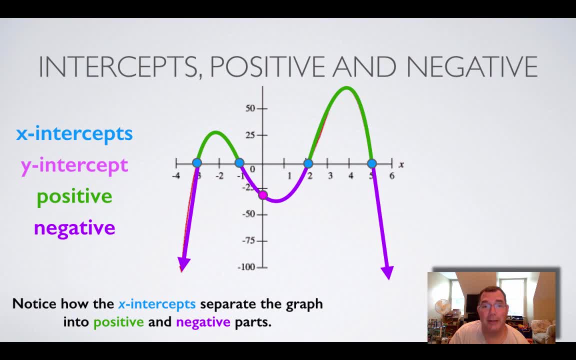 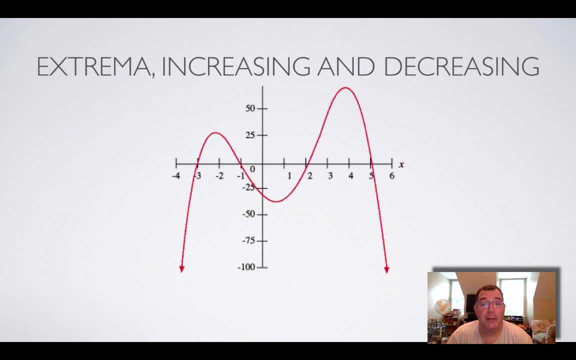 dot. What that means is the x-intercepts separate the graph into the positive parts and the negative parts. Okay, so now we have extrema maximums and minimums and we talk about increasing and decreasing. So the maximums are the tops of the hills, which are right here, because the graph 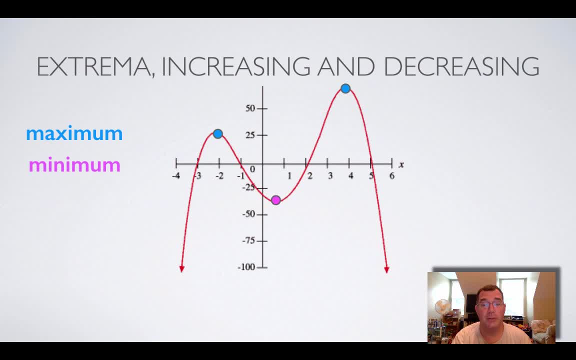 goes up and then goes down, And then the minimum. there's only one of those at that pink point right there and that's where the graph goes down, and then it goes down, And then it goes up, and then it comes back up, Increasing. remember we're reading from left to right, so any time the graph goes up, 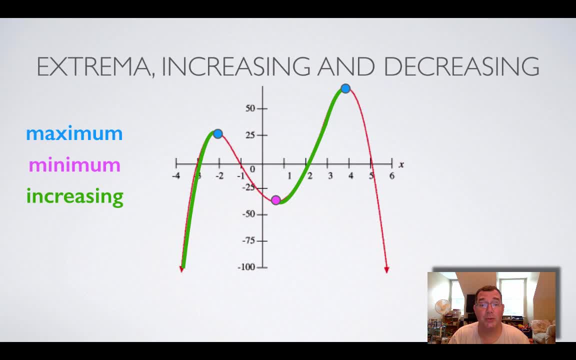 and to the right. that is where it is increasing. So I've labeled those with green curves and then any spot where it's going down and to the right we consider that decreasing. and I've labeled those with purple And, just like the x-intercepts, separated the function from the positive parts. 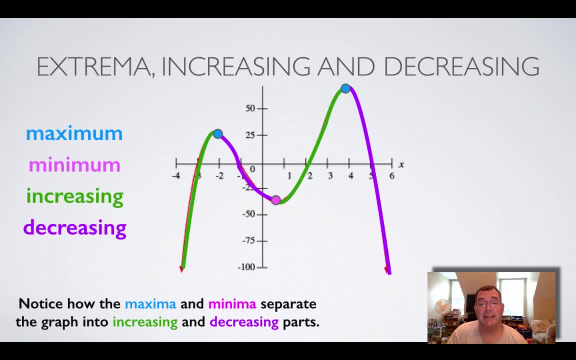 and the negative parts. the blue dots and pink dots separate the green and purple areas. So in other words, the maximums and the minimums separate the x-intercepts from the positive parts, and the green dots separate the graph into the parts where it's increasing and decreasing, And then finally, 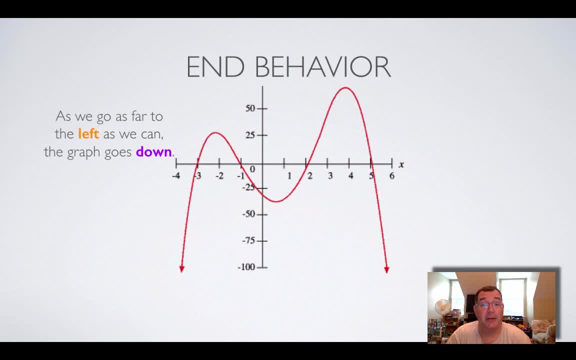 n-behavior. we're just looking at what goes on at the very, very left and the very, very right, So it can level off, it can go very, very up or it can go very, very down. So notice as we go very, very. 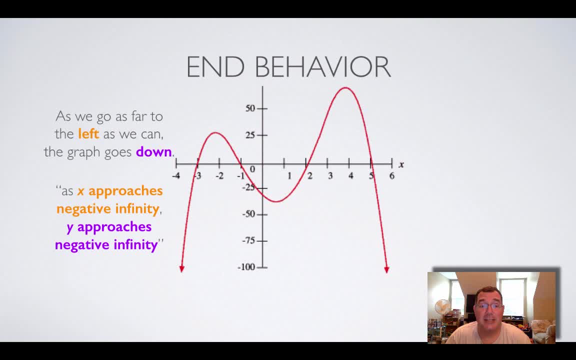 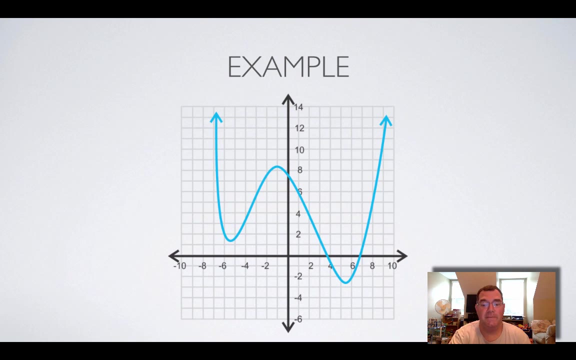 far to the left, the graph goes down and we say that as x approaches negative infinity, y approaches negative infinity. And then, as we go very, very right, the graph also goes very, very down. So as x approaches positive infinity, y again approaches negative infinity. So here's a final example. 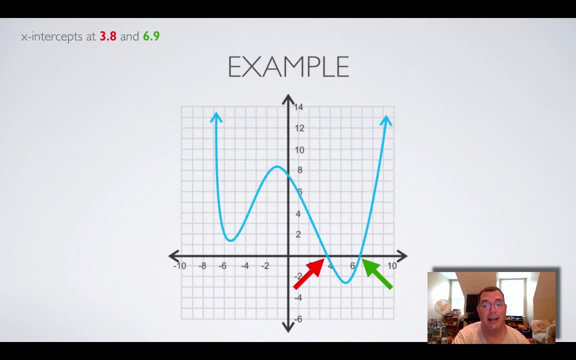 We've got x intercepts at 3.8 and 6.9.. That's where it crosses the x-axis. We have a y-intercept at 7.5.. That's where it crosses the y-axis. We have a positive function for x's that are less. 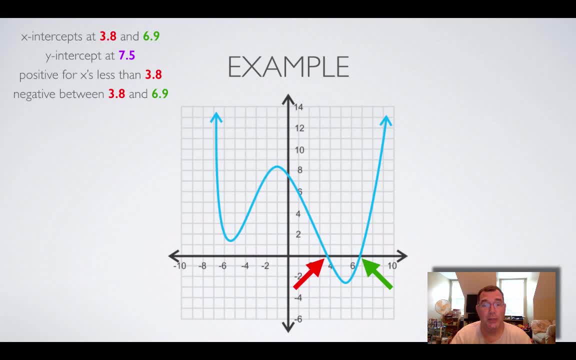 than 3.8.. We have a negative function between 3.8 and 6.9, and then we have positive x's, Um, we have a positive function for x's that are greater than 6.9.. Now, talking about maximums and 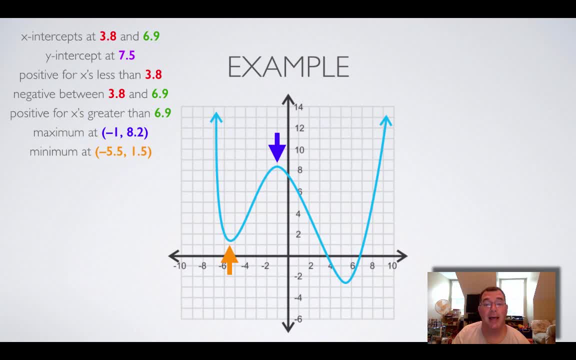 minimums. I have a maximum at negative 1 and 8.2.. I have a minimum at negative 5.5 and 1.5, and I have a minimum again at positive 5.5 and negative 2.5.. The function decreases before I. 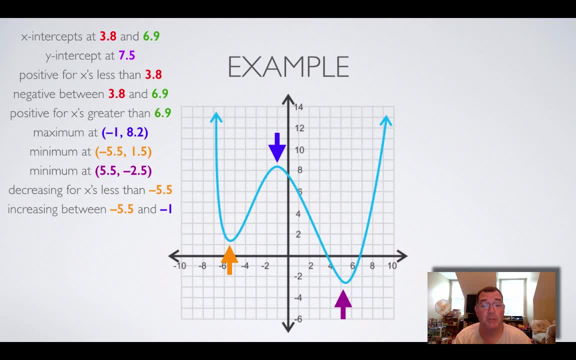 get to negative 5.5.. It increases between negative 5.5 and negative 1.. It decreases again between negative 1 and negative 2.5.. I have a minimum at negative 5.5 and 1.5.. I have a minimum at.